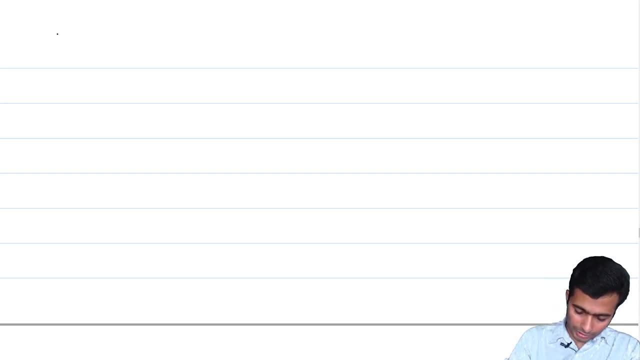 for these operators. So let us begin. So let me just write the. So let us begin. So let us begin. So let us begin with the heading spectral theorem. So suppose, before we enter into the statement of the spectral theorem, So if T be a linear operator on an inner product, 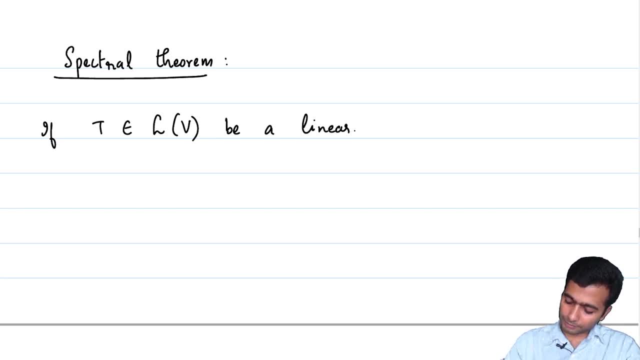 space be a linear operator on a finite dimensional inner product space. And suppose we have an orthonormal basis. And suppose beta is an orthonormal basis consisting of eigenvectors of T. This is called canonical comfort. So if T be a linear operator on 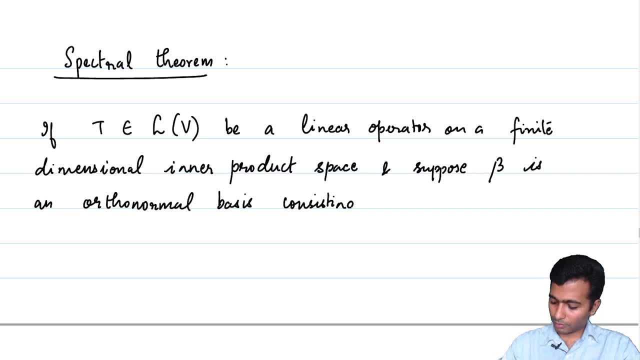 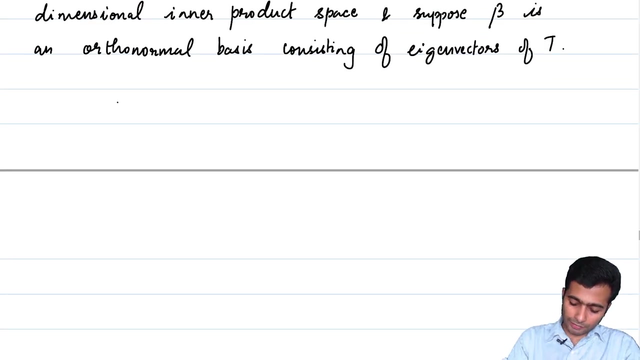 T, suppose we are in this setup. So observe that what we are demanding is that what is given to us is that T is a diagonalizable linear operator. not only that, the eigenvectors are orthonormal to each other. Then recall that the matrix of T with respect to beta. 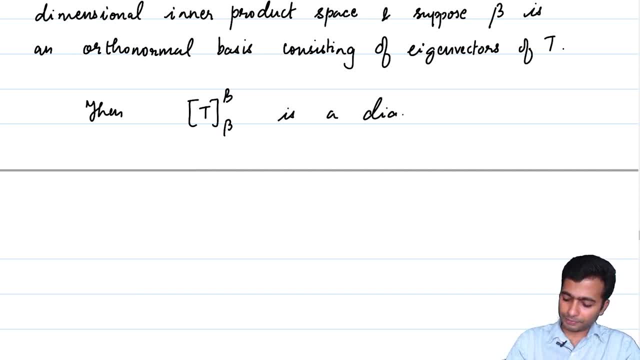 will be a diagonal matrix. What have we checked about diagonal matrices? We have seen that diagonal matrices are normal. The product of the diagonal matrix and its conjugate transpose will be equal to the product of the conjugate transpose of the matrix and the matrix itself. 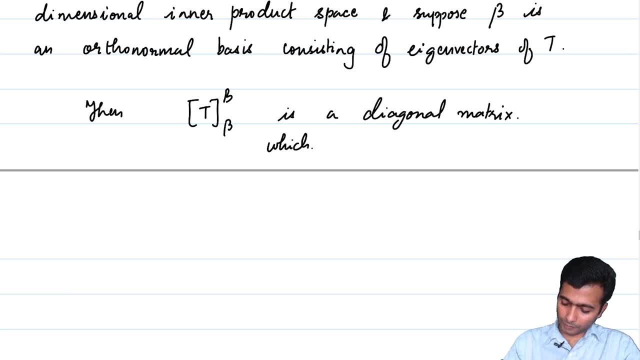 So, which is a normal matrix, And by one of the theorems we have proved earlier, If a linear operator has a matrix representation with respect to some orthonormal basis which will give us a normal matrix, then the linear operator itself is normal. This helps us conclude. 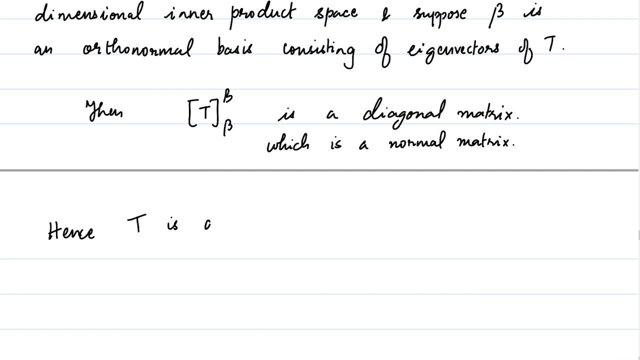 that T is itself a normal operator. So what we have observed is that if there is a diagonalizable matrix with a basis, If there is a basis consisting of orthonormal vectors, of eigenvectors, then the linear operator T is normal. Our spectral theorem is in some sense of converse to this. What our spectral 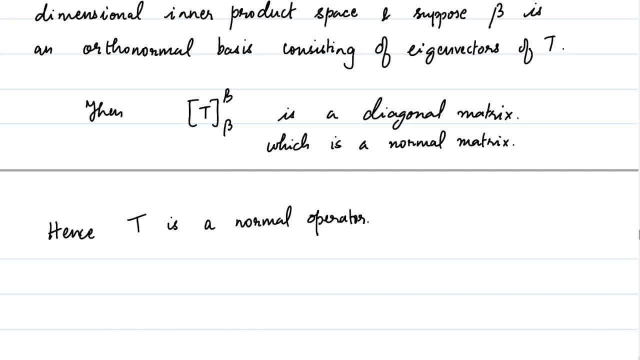 theorem says: is that in this is true? in general, spectral theorem says the following: If we start off with complex inner product space, finite dimensional complex inner product space, v, And if T is a linear operator, then our spectral theorem says that, in general, if we have a 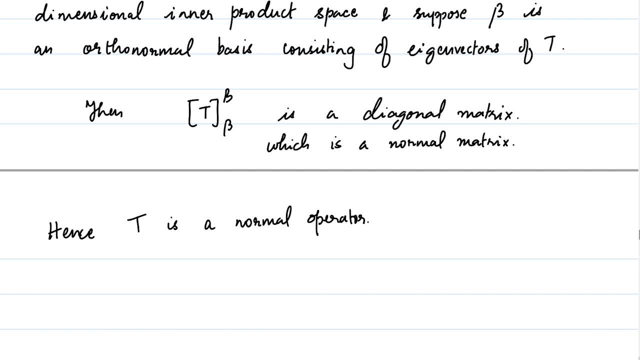 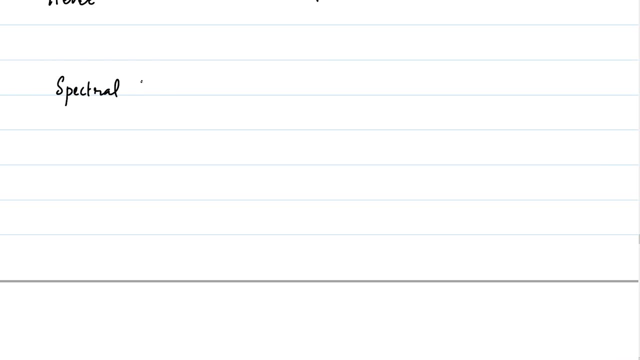 linear operator on V, which is normal. then there exists an orthonormal basis of V consisting of eigenvectors of T. In particular, our linear operator T is diagonalizable Spectral theorem for normal operators. So the setup has already been laid out for you. We are in a complex 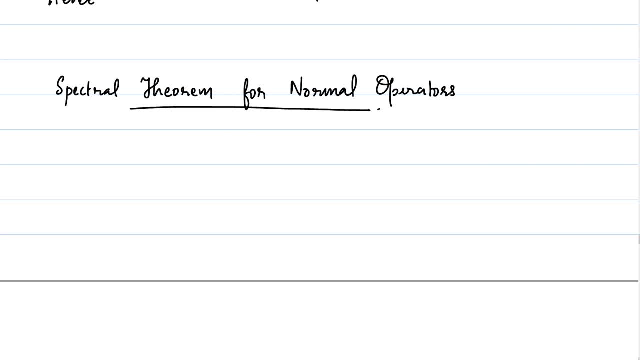 inner product space, finite dimensional complex inner product space and T is a normal operator on V. So let V be a finite dimensional operator on V. So let V be a finite dimensional operator on V. complex inner product space And T in L of V be a normal operator linear. 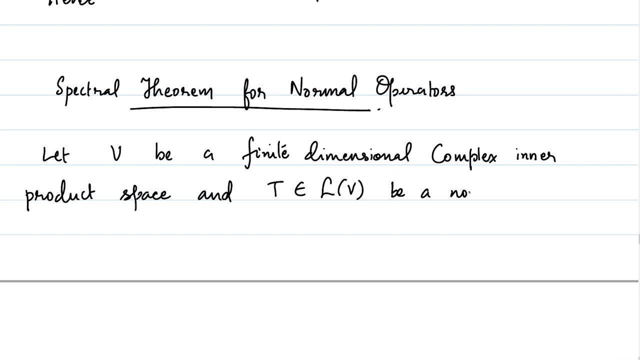 transformation from V to itself be a normal operator, Then the spectral theorem tells us that then there exists an orthonormal basis of V consisting of eigenvectors of T. So the spectral theorem tells us that not only is it diagonalizable, but the basis of eigenvectors of T they are. 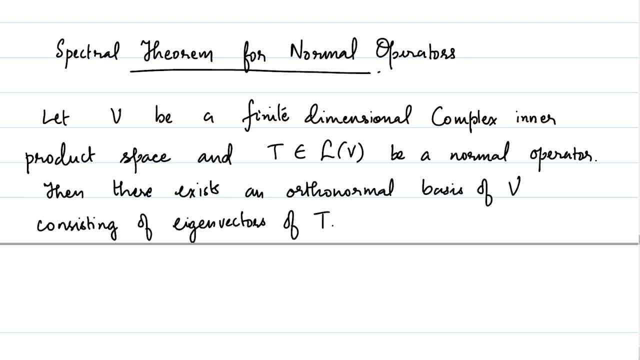 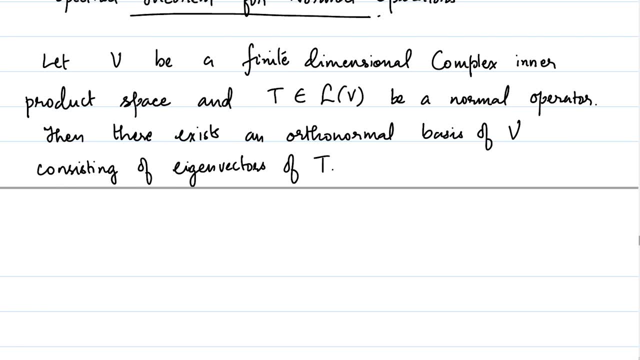 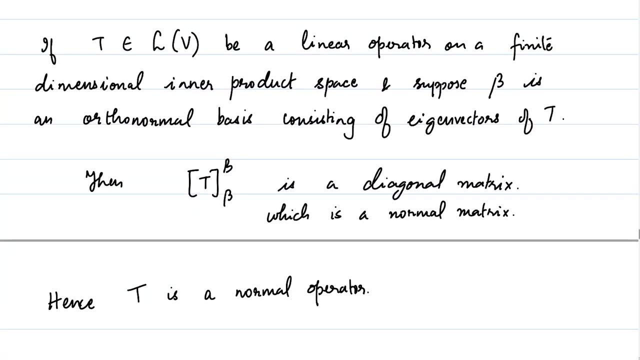 also orthonormal. So let us give a proof of this. before giving a proof of the spectral theorem, Let us look at what we have actually observed right now. What we have just seen is in the previous observation. the previous observation here was telling us that if you 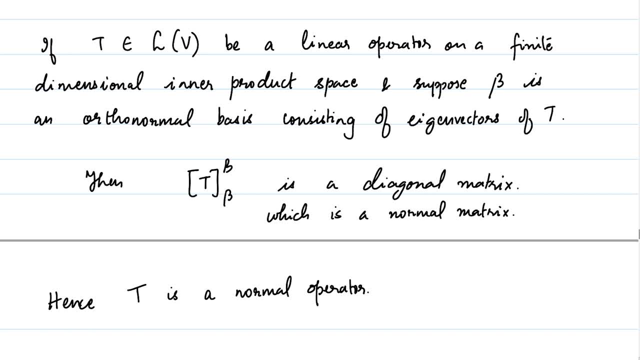 have a linear operator which satisfies the condition that V has an orthonormal basis consisting of eigenvectors of T, then T is necessarily a linear operator on V. So let us give a proof of this. So we can assume that that T is essentially a normal operator And the spectral theorem 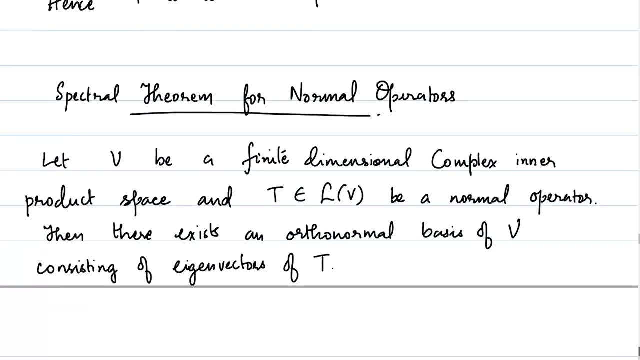 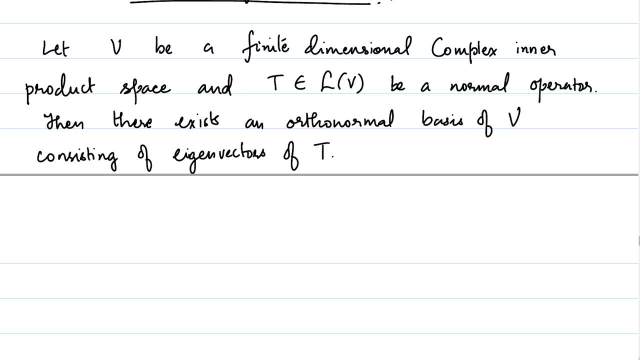 tells us that if T is normal, then V consists of. V contains an orthonormal basis consisting of eigenvectors. So in a complex inner product space, normal operators are precisely those operators which has which satisfies the condition that V has an orthonormal basis. 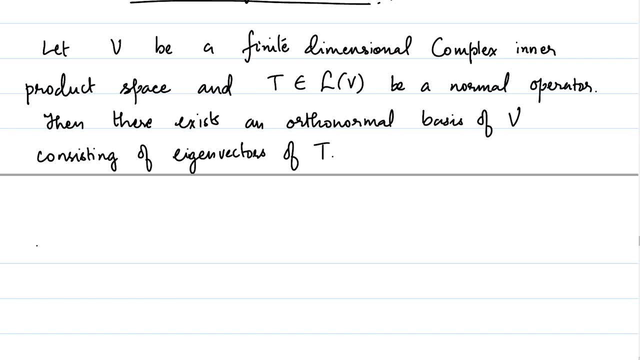 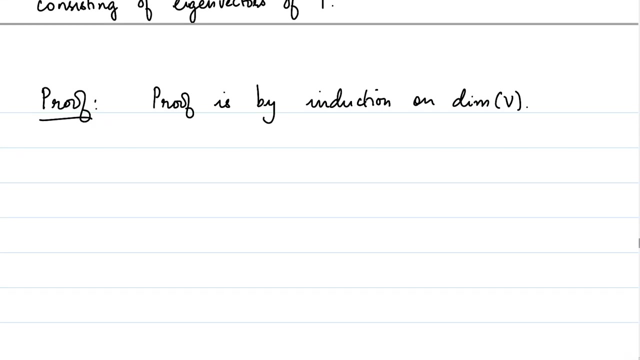 consisting of eigenvectors of T. So let us give a proof of the spectral theorem. So The proof is by induction. induction on what? Induction? on dimension of V. So this is a very finite dimensional inner product space proof that we are going to get. So when which? 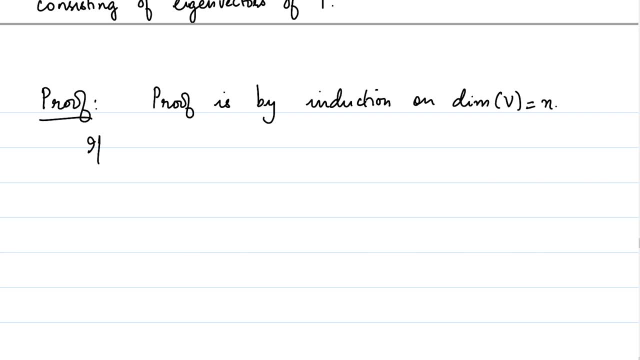 let us call it to be equal to n. So if n is equal to 1, what does that mean? That means that let V be basis of capital V, which has norm 1, such that length of V is equal to 1.. So since capital V has dimension 1, this particular vector will form a basis. and because 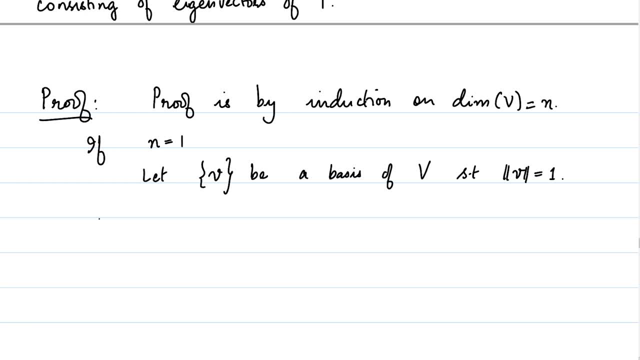 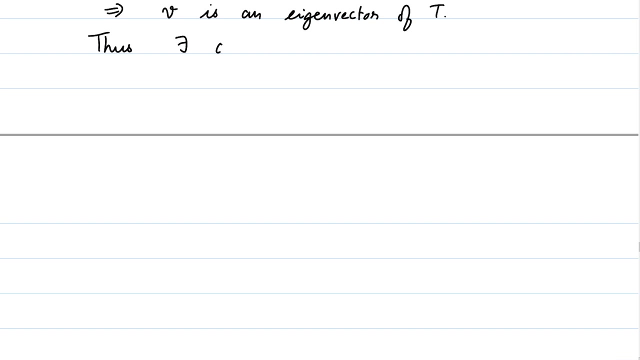 there are no other vectors, it is, by default, an orthonormal basis. We know that Tv is a scalar multivariate vector, So this is the principle of V, since V is a one-dimensional vector space, And that implies that V is an eigenvector of T, And thus there exists an orthonormal basis consisting of V. 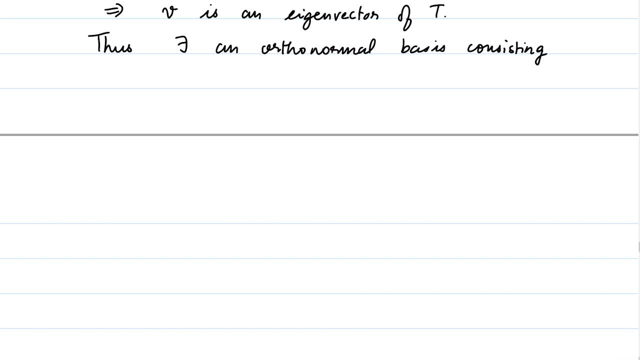 So, that is, when n is equal to 1, there is nothing to prove. Let us now assume that n is greater than 1.. So by induction hypothesis, let us assume that the theorem has been proved for up to n minus 1.. By induction hypothesis, assume: 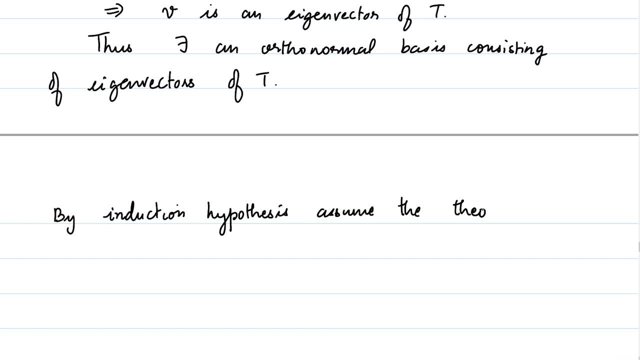 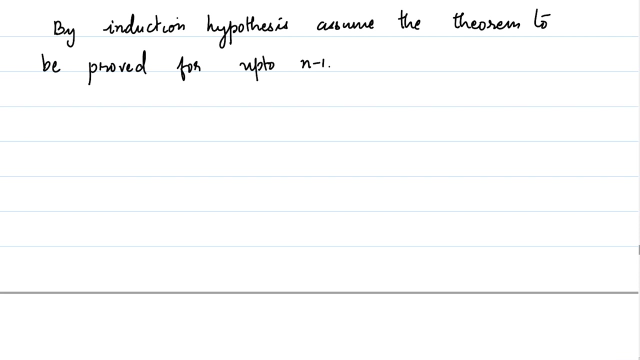 the theorem To be proved for up to n minus 1.. So we will prove that when dimension of V is equal to n, then the spectral theorem is satisfied, or spectral theorem is true. So the induction hypothesis tells us that for any linear operator, 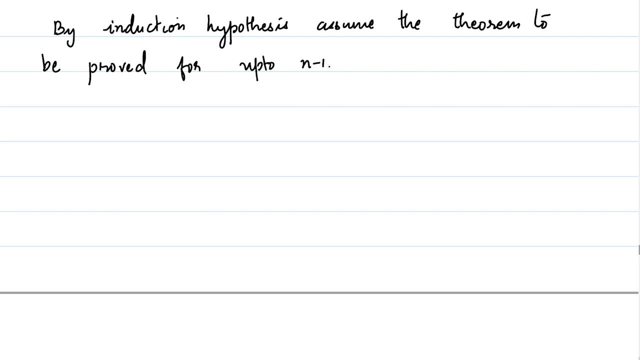 Which is a normal operator, on a vector space, which is a complex inner product space of dimension less than n, up to n minus 1, there exists an orthonormal basis consisting of eigenvectors. So to prove for n, let us consider the characteristic polynomial of our given operator. So let 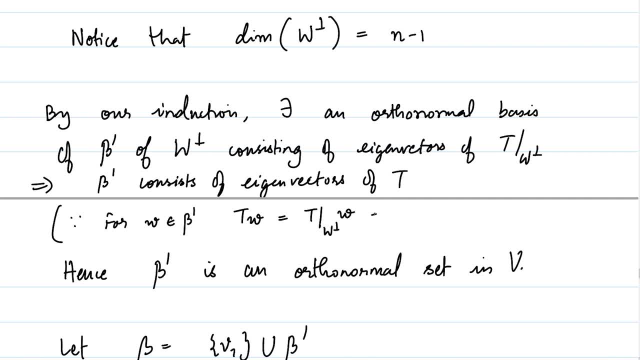 to the orthogonal complement of w acting on W, and this just going to be some lambda times W. W is an eigenvector that I have just noted. That would imply that each of the beta prime consists of eigenvectors of T as well. Well, eigenvectors of T restricted to W orthogonal. 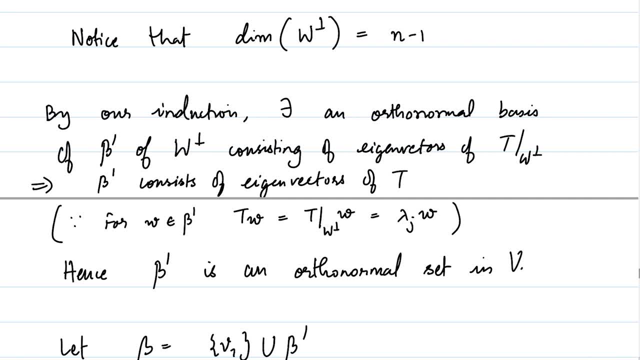 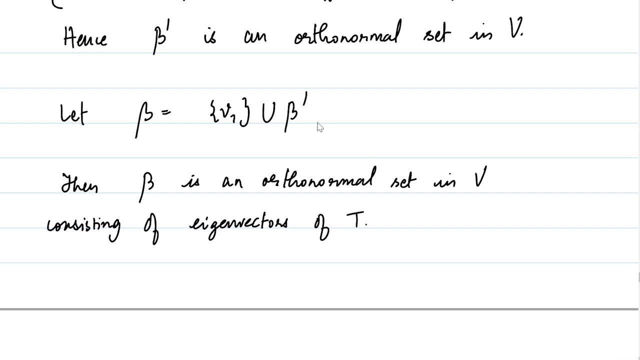 is just going to be eigenvectors of T as well. So that is the simple observation here, And therefore this beta will have an orthonormal set consisting of eigenvectors of T. But what is the size of beta? The size of beta is equal to n minus 1 plus 1, which is equal to n, because 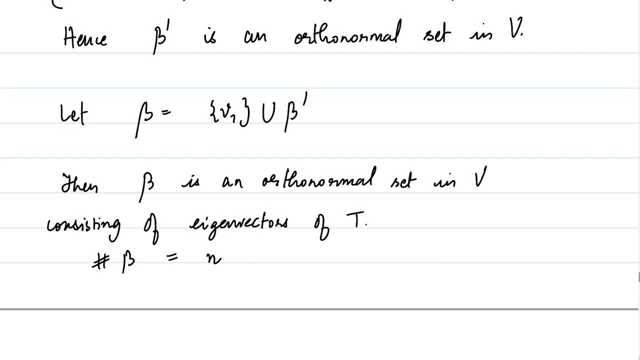 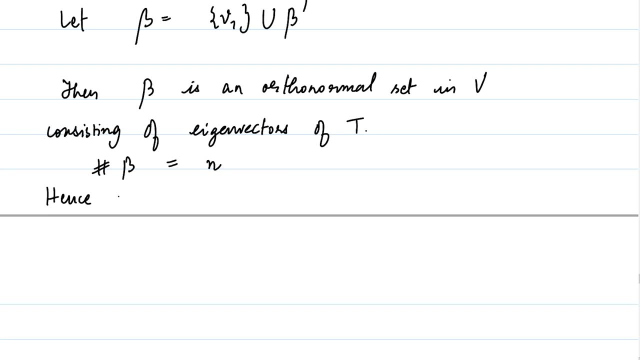 beta prime has n minus 1 vectors. After all, W orthogonal had dimension n minus 1. And they are all. that is an orthonormal set. Hence, beta is a set of size n Which is linearly independent. And what do we know about linearly independent set of? 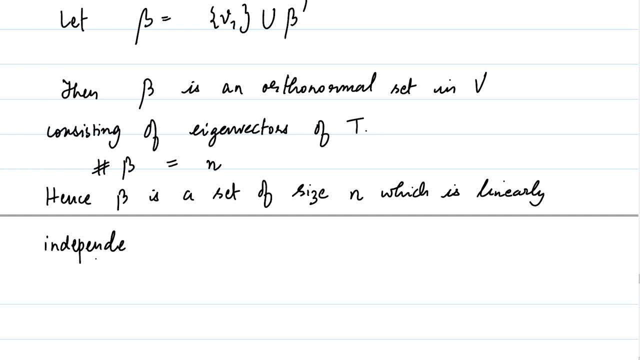 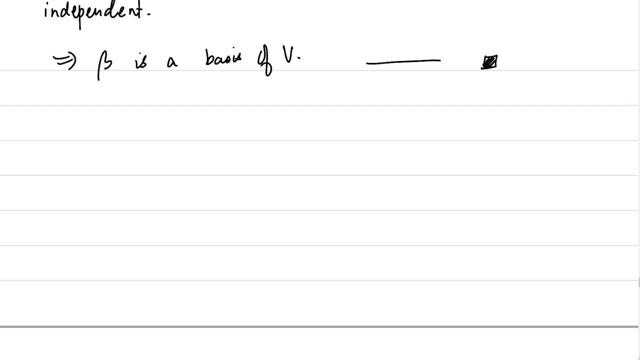 size n in a dimension n vector space. We know that it is a basis. This gives that beta is a basis of V And we are done with the proof. So we have just proved that in a complex inner product space a normal operator is always diagonalizable, not orthogonal. So 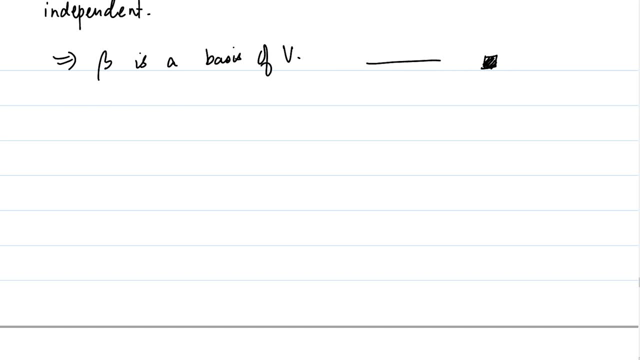 not only is it diagonalizable, we also have a basis of eigenvectors which is orthonormal. That is pretty nice. So there are a couple of observations, couple of remarks here. The first one is to observe that this is a statement which has complex inner product space put. 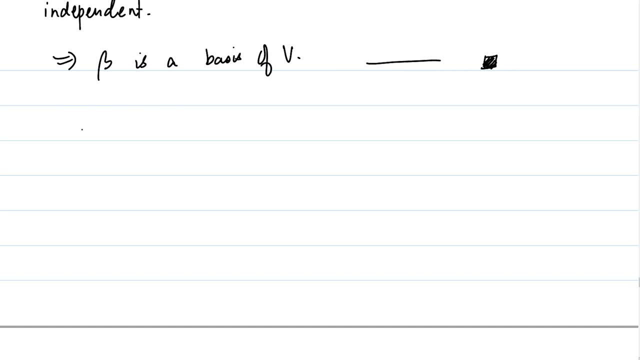 into the very hypothesis of the statement, because if you consider T, so remark, consider T from R2 to R2, this is a real inner product space given by T of x, comma, y to be equal to. let us look at the example we had given in one of the previous lectures. we will just 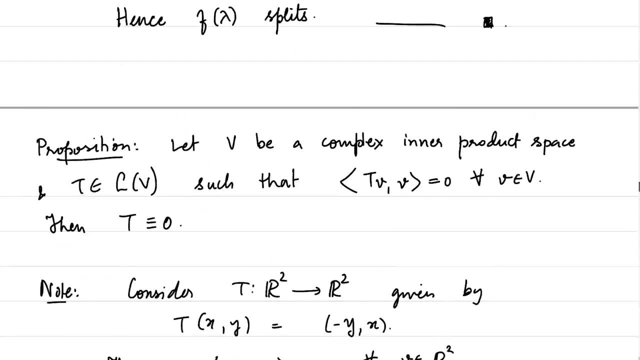 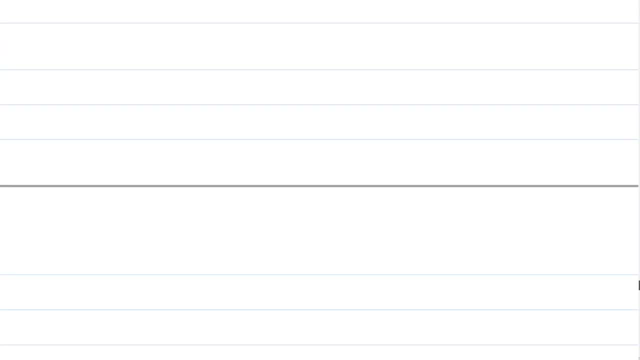 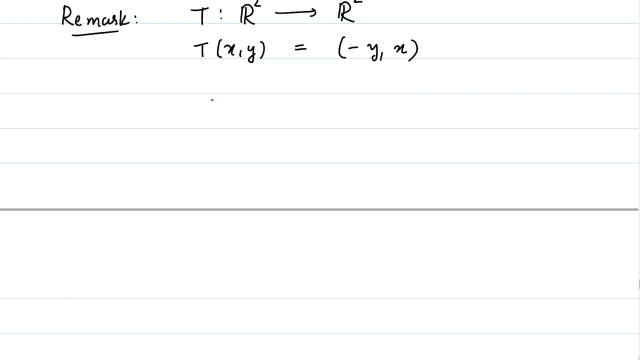 use the same example here. Was it x minus y, Yes, T minus y, Yes, T minus y comma x? let us look at this particular example: Minus of y comma x. So what was the characteristic polynomial To do that? let us look at what was T, beta, beta, where? 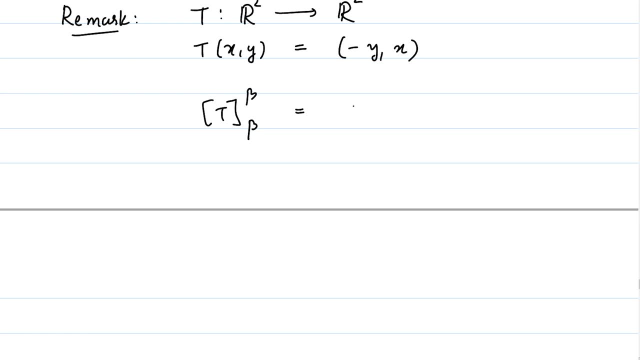 beta was the standard basis, If you recall. this is just going to be equal to 0, 1, minus 1, 0.. And hence f of lambda is just going to be equal to lambda square plus 1.. And if 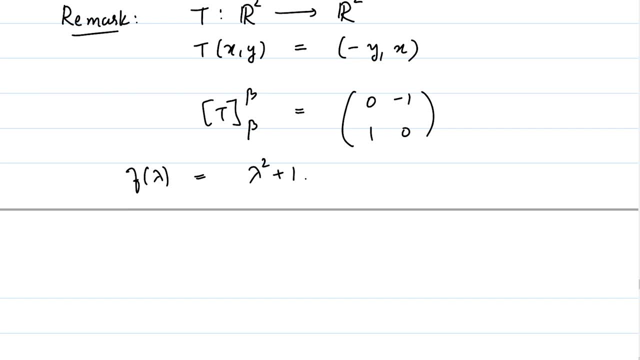 you notice, this is an anchor. Notice: this is a polynomial which does not split over real numbers, does not split over r. So the fundamental theorem of algebra is: it tells us that it splits over the complex numbers. This particular polynomial, however, does not split over r And hence this is 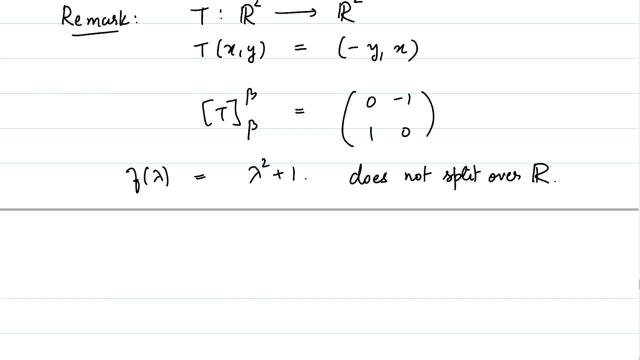 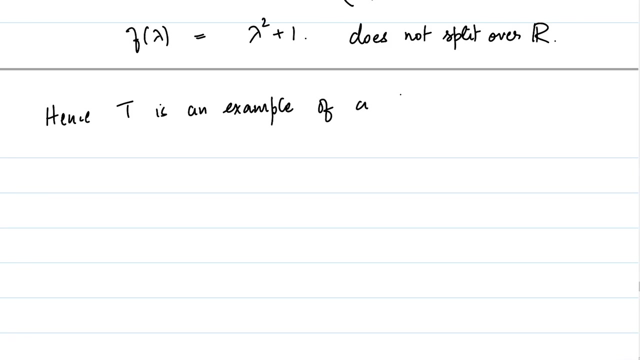 a linear operator which does not even have eigenvalues: t from r 2 to r 2.. So it is a normal operator which does not even have eigenvalues. So there is no question of getting hold of a basis consisting of eigenvectors. So hence, T is an example of a normal operator. 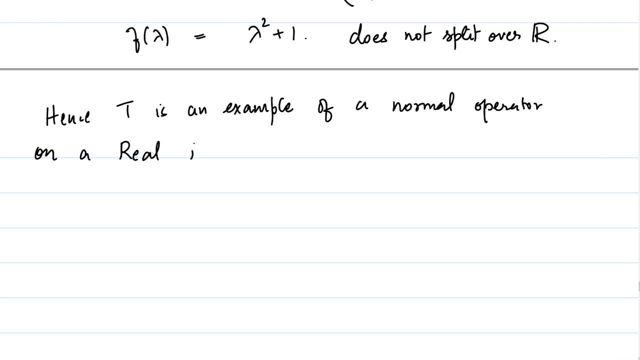 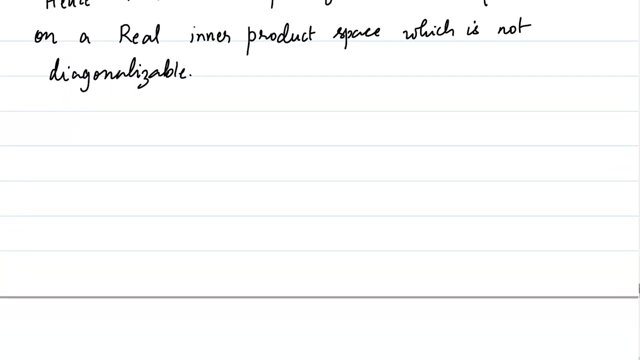 on a real inner product space which is not diagonalizable. Let us look at, however, the case when, let us say, call it S. So let us look at example now: S b, from c 2 to c 2, very similar map. let us define: 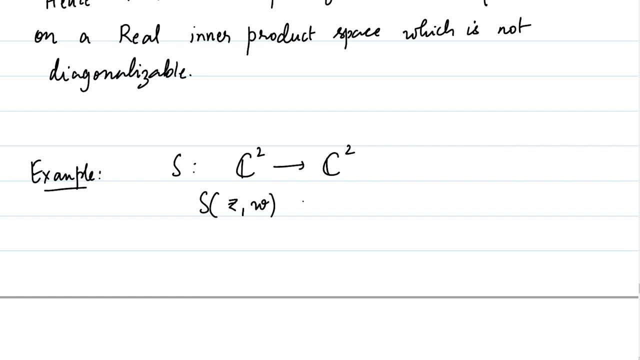 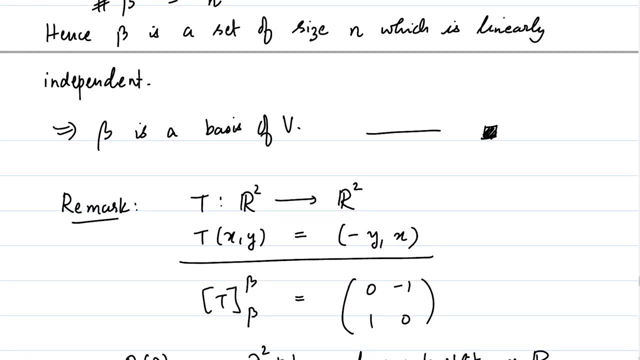 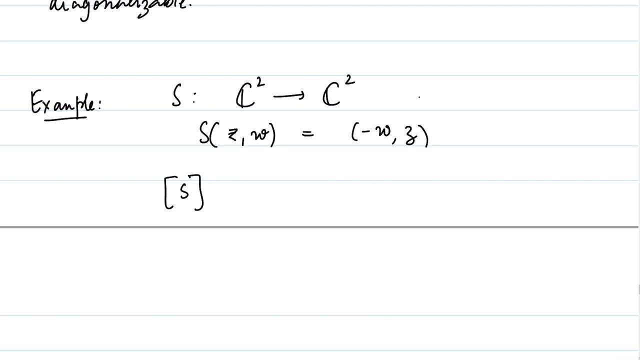 S of. instead of x comma y, let us use some z comma w, and this will be what minus of t. So w comma z, just like the map we have defined here. And let us see what will be the matrix of S with respect to beta. So let beta be equal to the ordered basis consisting of 1,. 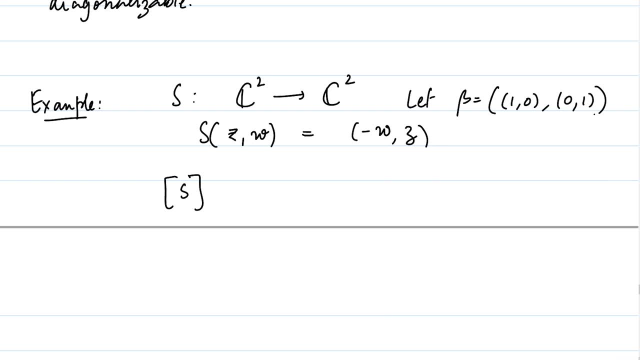 0 and 0, 1.. Notice that this is in C 2.. So all complex numbers. you look at the span with respect to all the field of scalars being complex numbers. Okay, So what is S? beta? beta, As was observed earlier, this is just going to be equal to 0 comma. 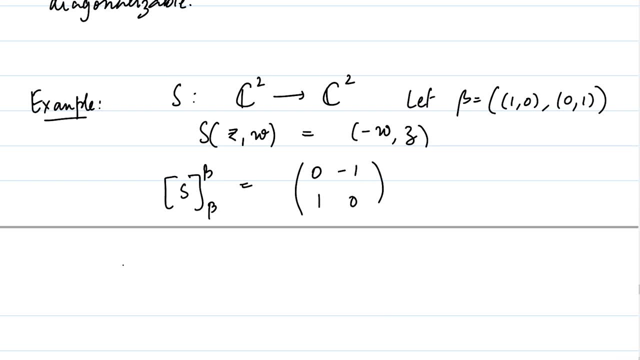 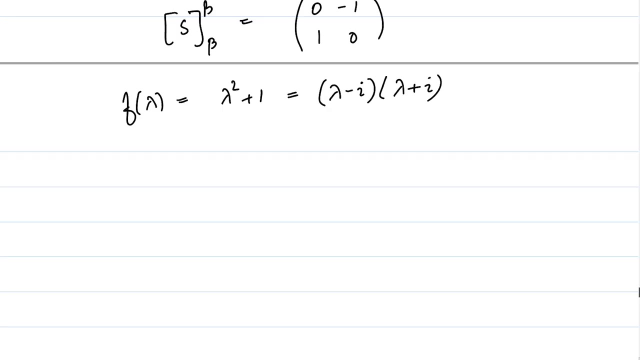 1 in the first column and minus 1 comma 0.. And therefore f of lambda is equal to lambda square plus 1, which is lambda minus i times lambda plus i, where i is the square root of minus 1.. Therefore there are two eigenvalues here. hence lambda 1 is equal to i and lambda 2. 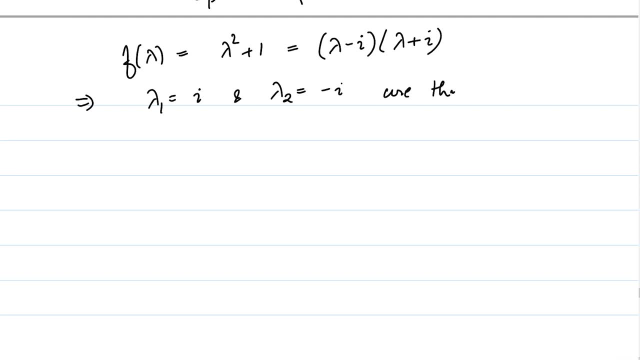 is equal to minus i are the eigenvalues. So notice that the split is to be expected by the fundamental theorem of algebra here. in this case it was easy. hence I could write it down very easily: Lambda 1, the roots are going to be the eigenvalues of our linear. 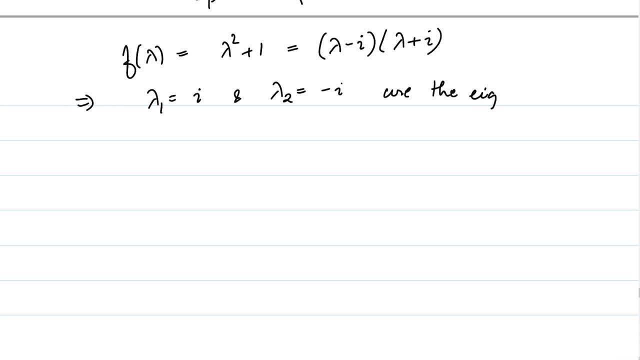 operator. So i and minus i are the eigenvalues of T of S. rather That means S of. let us look at what the eigenvectors will be at for: eigenvector of Z of i. Eigenvector. 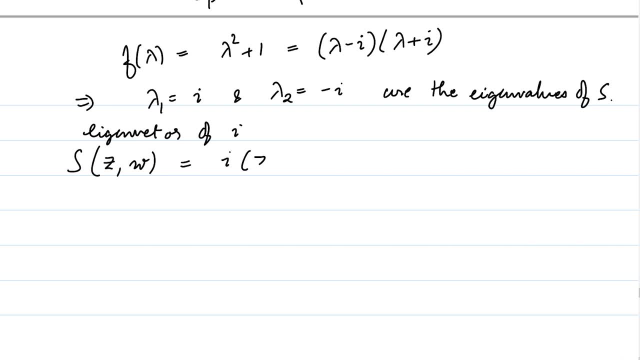 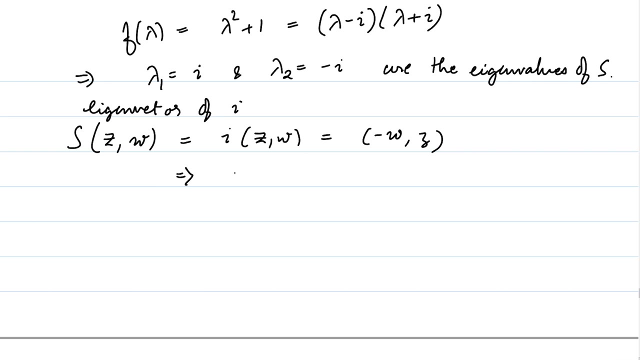 one of the eigenvectors of i will be something of this type: i times Z, W, but this, we know, is equal to minus of W comma Z. yes, That means this is equal. that mean this gives us that I Z L. 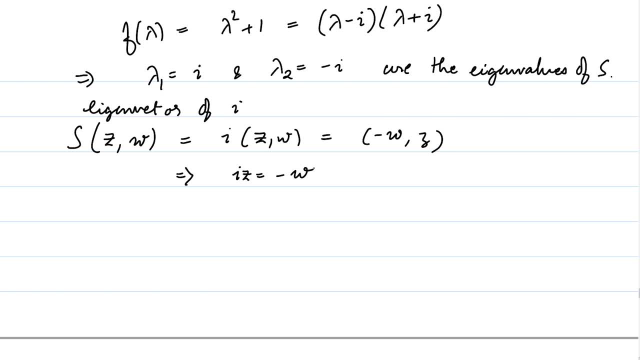 I set V to equal. I set V to equal is equal to minus of w. So this would imply that when z times the first one can be put as 1, if z is 1, w would be minus i. This is an eigenvector of e, responding to i eigenvalue. 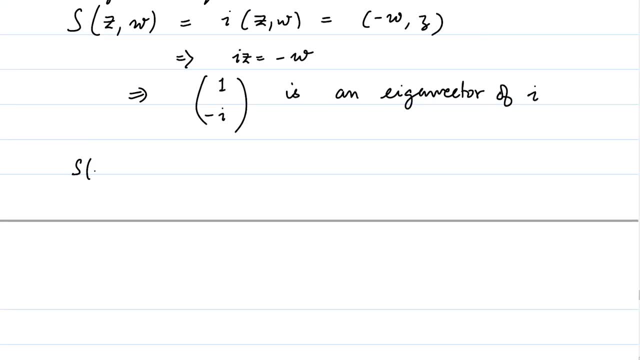 lambda 1 equal to i. How about minus i? If s of z comma w is equal to minus of i times z comma w, this would imply that i times z is equal to w and minus of i times w is equal to z, which makes sense. 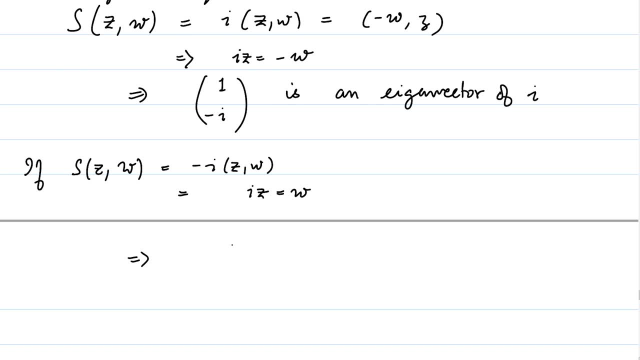 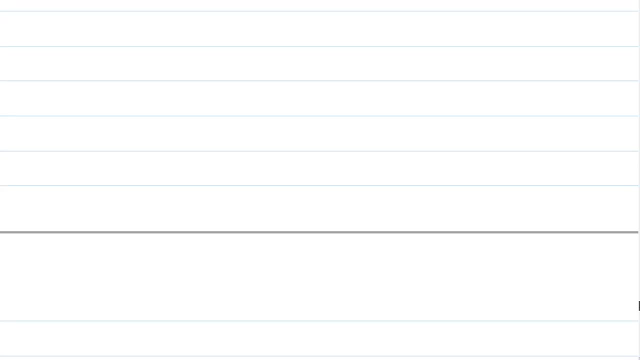 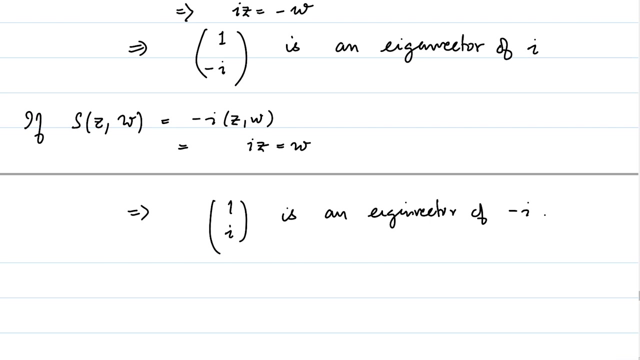 And therefore z is equal to 1 comma. i is an eigenvector of minus i, So what would be an orthonormal basis? So we have already seen that in the case of a normal operator, the eigenvalues corresponding to distinct eigenvectors corresponding to distinct eigenvalues should be orthonormal. 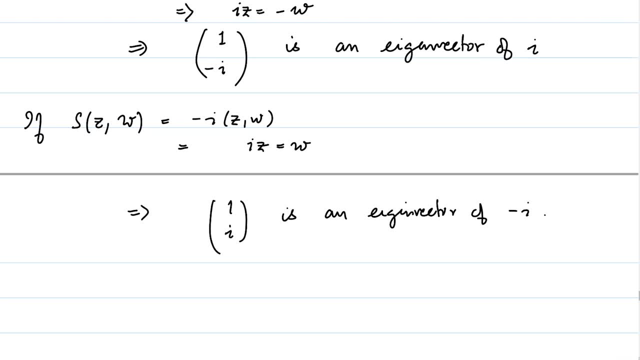 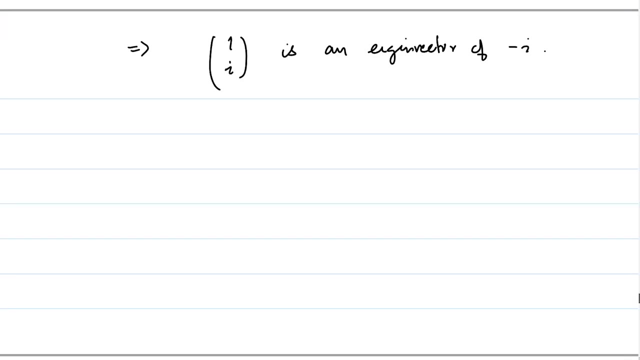 So, in particular, this is orthonormal. you can check it straightforward in a in a straightforward manner, using the inner product space as well. All right, So i am sorry. right. so beta being equal to 1 comma minus 1, after orthonormalizing. 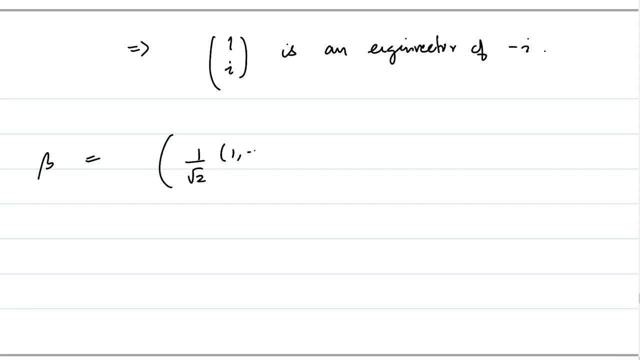 it will be 1 by root 2 times 1 comma minus i, and 1 by root 2 times 1 comma. i is 그냥 1.3.. Okay, an orthonormal set consisting of orthonormal basis, rather consisting of eigenvectors of. 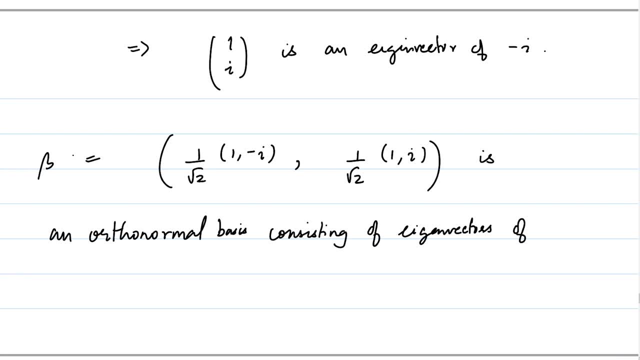 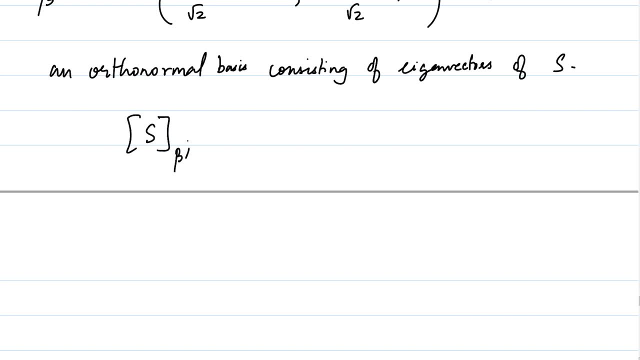 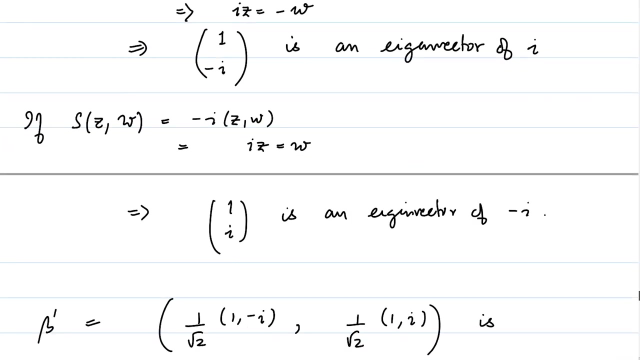 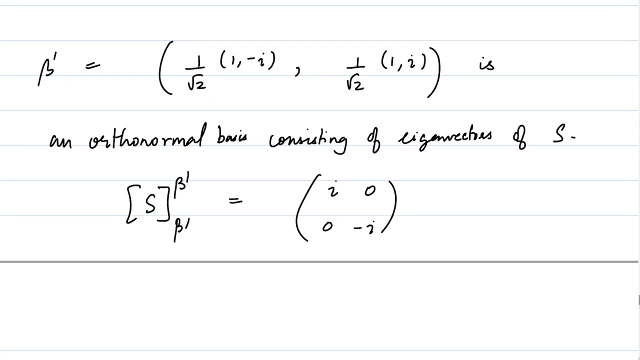 S. Let us call it beta prime. we already called beta as the standard basis of S, and what is going to be S, beta, prime, beta prime? this is just going to be equal to i comma 0, 0 comma minus i. So that is an example of this. example illustrates that in the case. 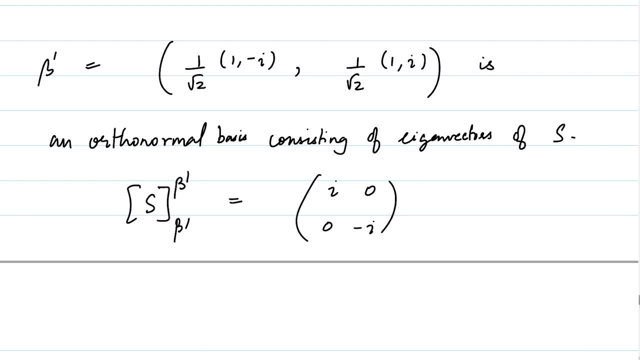 of complex inner product spaces, normal operators are diagonalizable, Whereas in the case of inner product spaces, normal operators need not be diagonalizable. The example we just gave illustrates that. However, if you notice, our first example was an example of a normal. 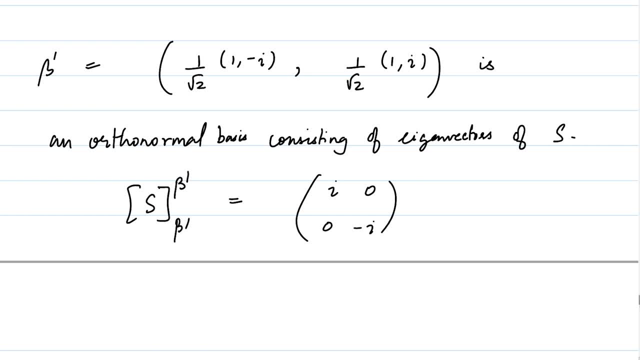 operator which was not a self-adjoint operator. So of course all self-adjoint operators are normal operators and therefore, if you consider self-adjoint operators over complex inner product spaces by the spectral theorem for normal operators, we know that that is. 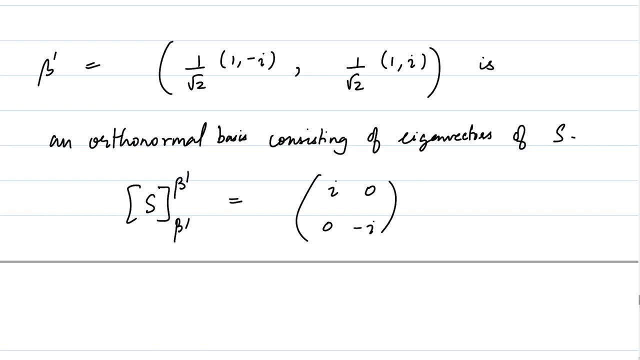 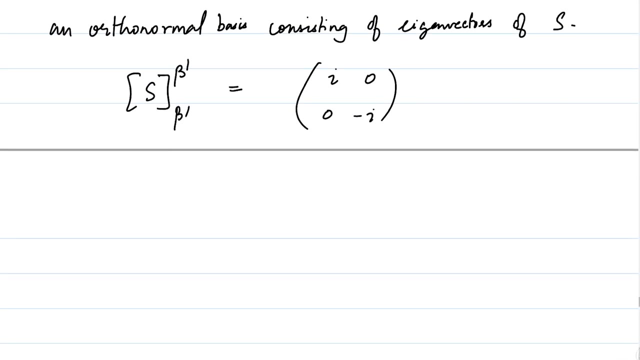 also a diagonalizable linear operator. But we can ask more. what can we? can we at all say anything about self-adjoint operators on real inner product spaces? The answer turns out to be yes, we can say something more, and that is going to be the content of the spectral theorem for the self-adjoint linear operators. 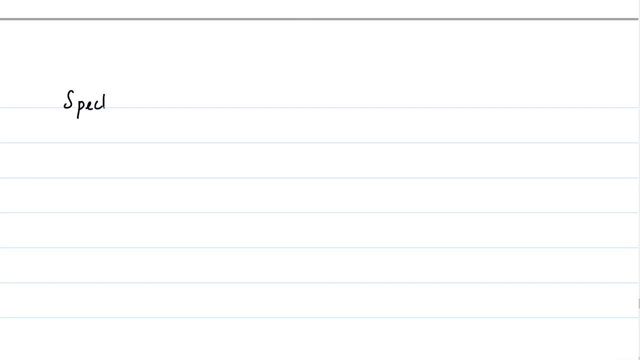 So this is going to be the spectral theorem of self-adjoint operators. So now let us look at a real inner product space. we have already addressed the case of a complex air product space. right, Self-adjoint operators are normal and, as I was just mentioning, 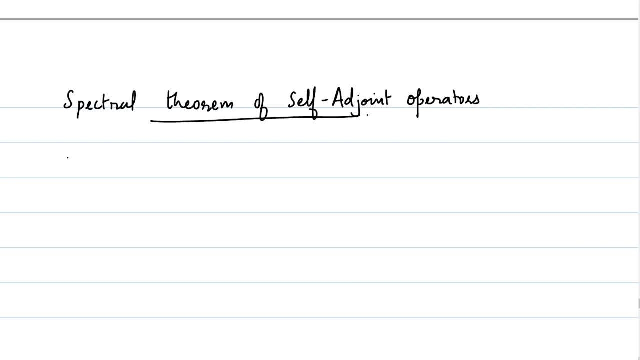 because of the spectral theorem for normal operators, we also have a spectral theorem for self-adjoint operators in the case of complex inner product space. Let us now look at a finite. enough in the complex product space based system. So now let us apply. 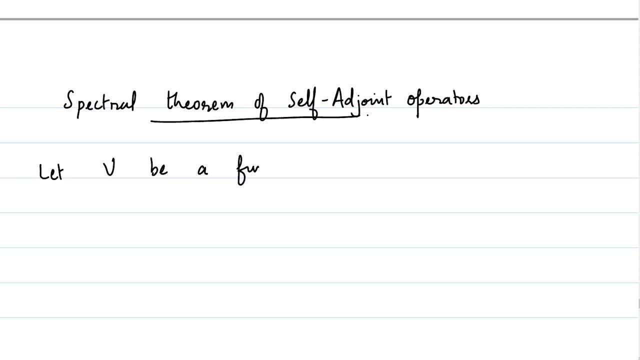 the spectral theorem of this kind of Hardy scale product to a range Due to normal operators, dimensional real inner product space. So the field of scalars in this case is the real numbers inner product space. Then, and T in L of V be a self adjoint operator Did. 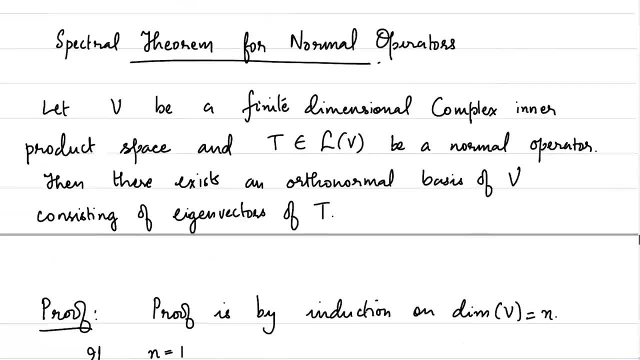 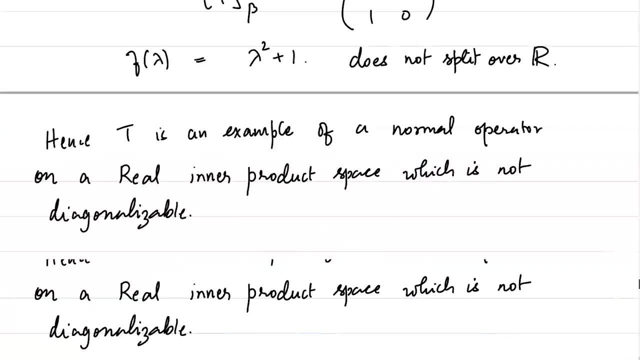 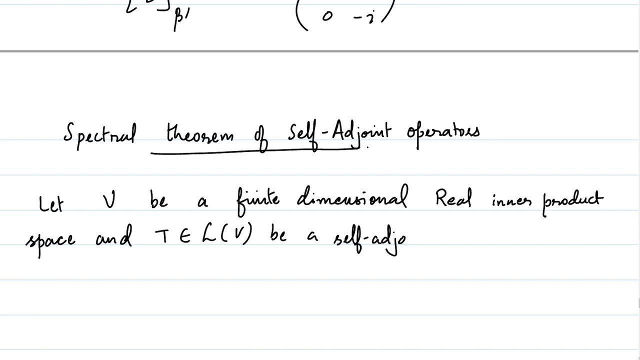 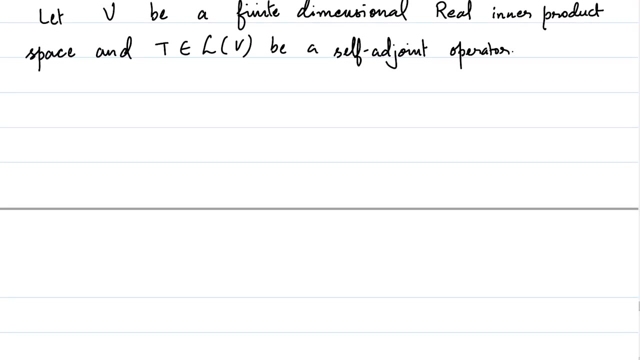 I mention in the statement of the spectral theorem above that T is normal. Yes, it is, it is mentioned. So in this case we are going to focus on T. in L of V be a self adjoint operator, Then their axis an orthonormal basis. 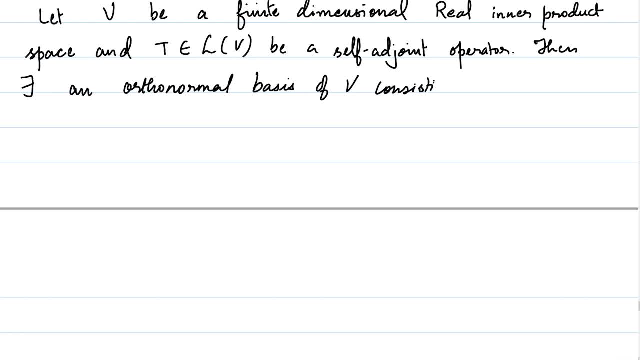 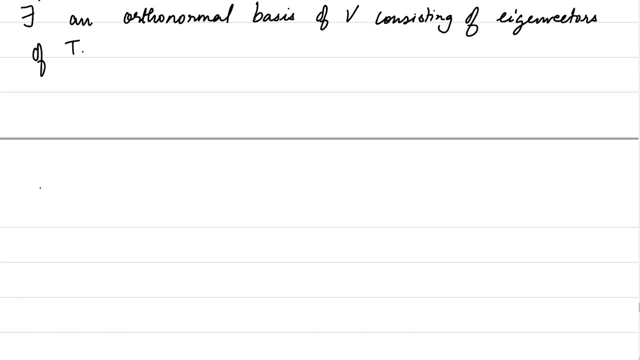 of v into L, of T, of L, consisting of eigenvectors of. so in the case of a real inner product space, if you are given a self adjoint operator- we do have that- it is diagonalizable over R. So we have already done all the major work. So let us give a proof of this. the proof. 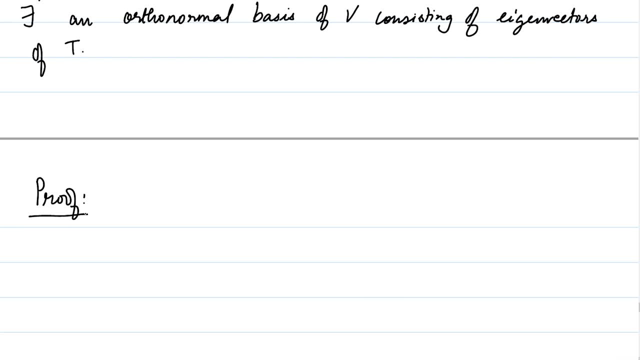 has already been done to a large extent already. The question would be: we will mimic the proof that we were trying to do in the case of normal operators? where would be the hurdle that would come? So recall that again, the proof can be done by induction. 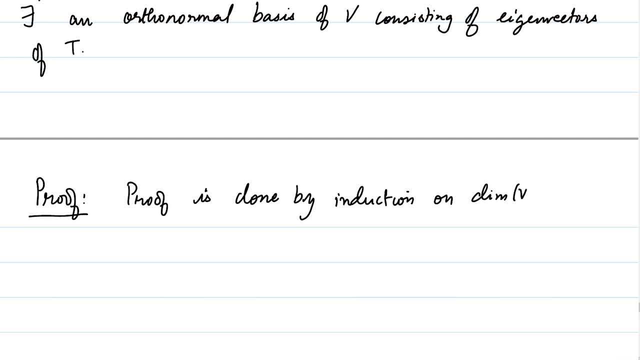 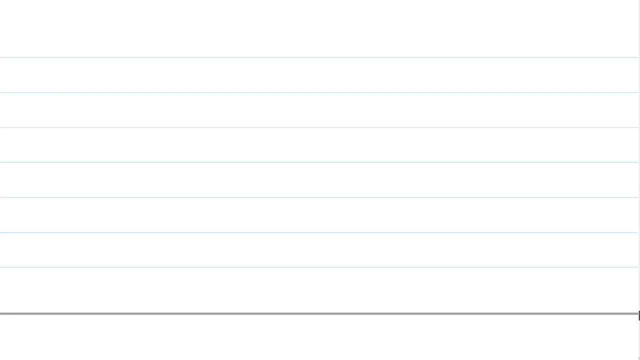 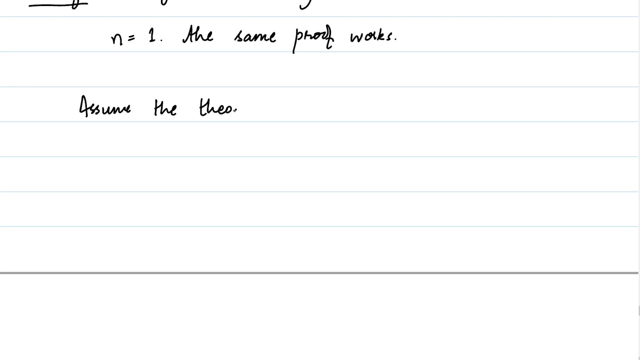 on the dimension of V, which is equal to n, n is equal to 1.. It is straightforward, is the same proof works? and let us prove. assume that the theorem has been proved up to n minus 1.. Now, if you are to mimic the proof of the spectral theorem, 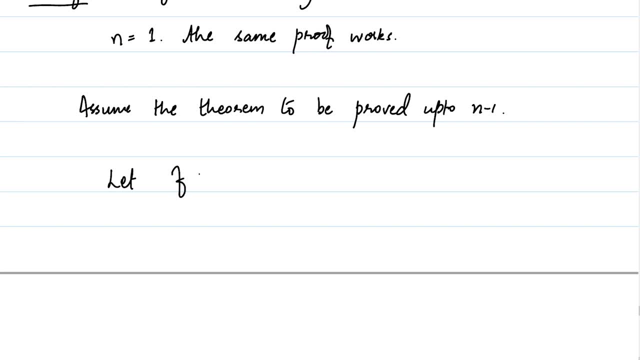 for normal operators, you can do this, So you can do this, So you can do this. So for normal operators, we will be considering the characteristic polynomial be the characteristic polynomial of E. However, now we are in a real inner product space and we will not be able to say that. 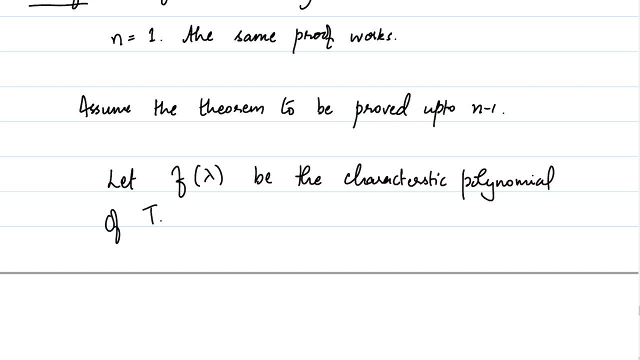 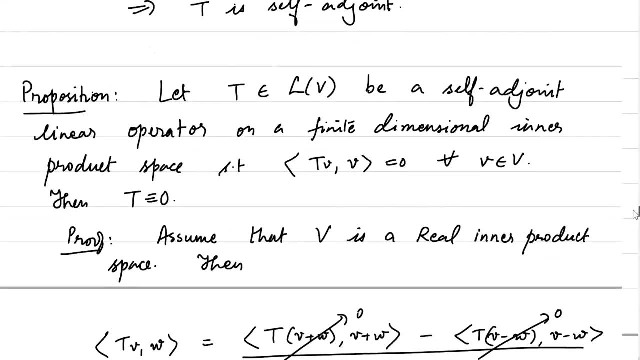 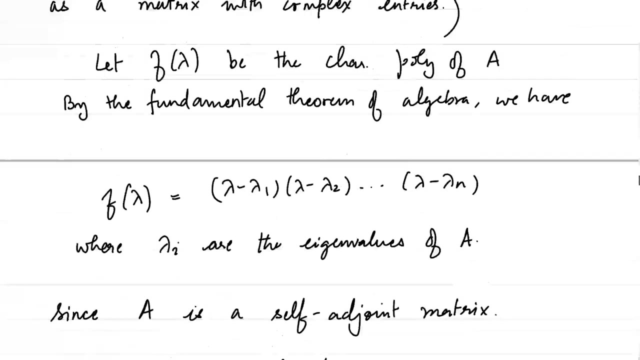 the characteristic polynomial splits over real numbers in the general case. However, let me go back to a recent example. So this is a result from your, from the previous lecture regarding the characteristic polynomial of self adjoint operators. Yes, this is precisely the statement. So notice that if it is a self, 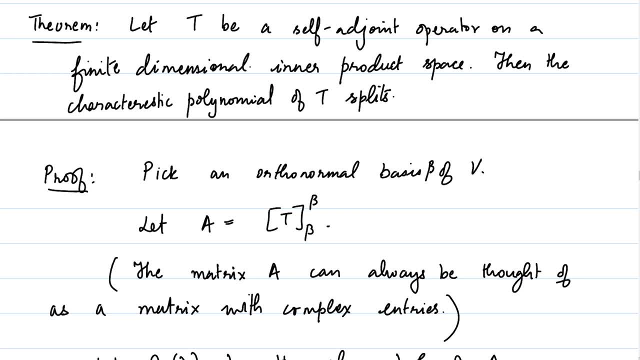 adjoint operator on a finite dimensional inner product space, whether complex inner product space or real inner product space. In the case of complex inner product space, this theorem is redundant because, anyway, fundamental theorem of calculus, fundamental theorem of algebra tells us that the characteristic polynomial space, in the case of real inner 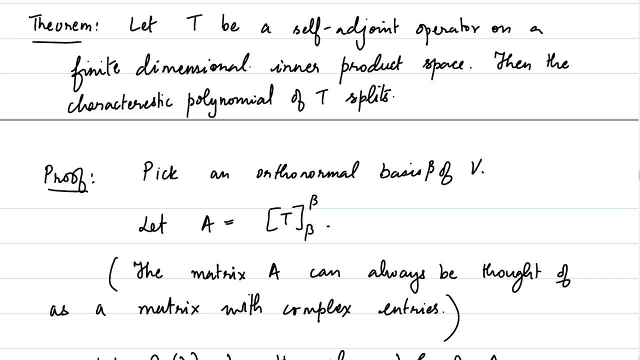 products is where this is telling us substantial amount of information. this tells us that it splits. So I did not actually mention over R, but that is understood Here. I did not write over R because the statement was more general. it splits over the field of scalar. So if it was in the case of a complex inner product, 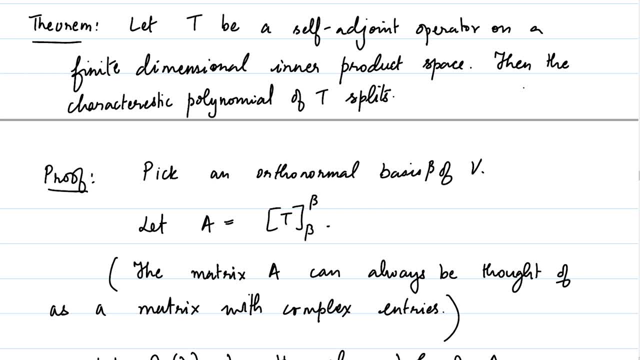 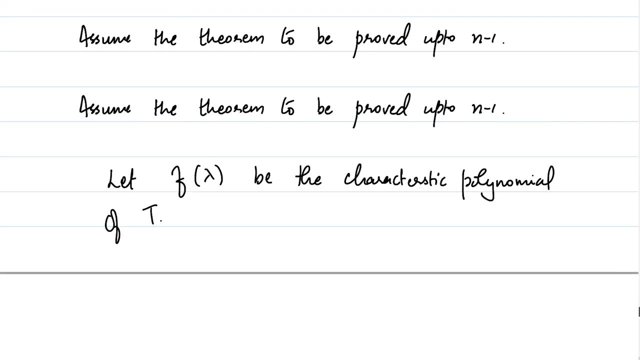 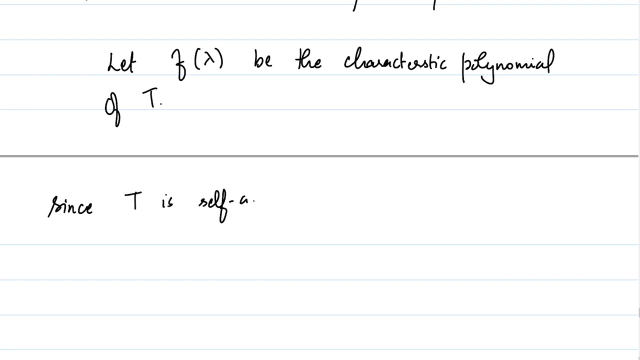 space. it splits over C- real inner product space. it splits over R. the proof did capture that, So I do not want to go through the proof again. but what it tells us is that splits over R because T is self-adjoint, So we will use that information. since T is self-adjoint, this is very important. 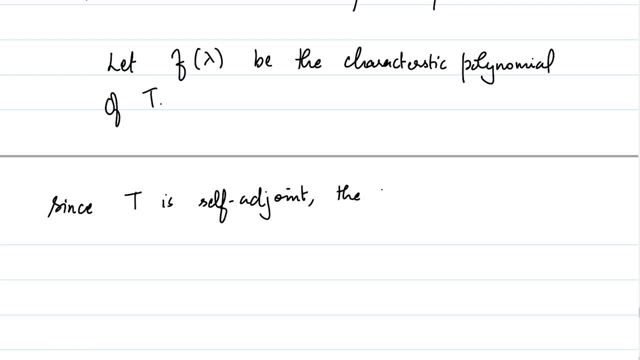 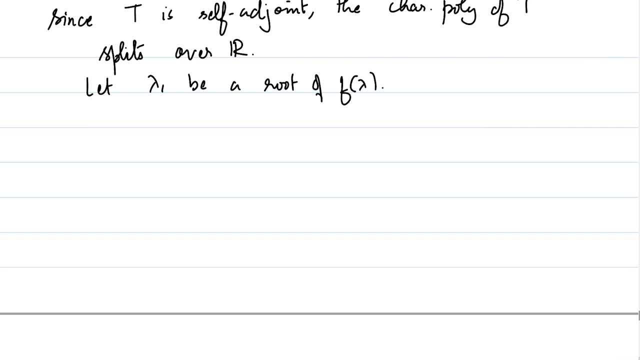 because it is self-adjoint, the characteristic polynomial of T splits over R, and let lambda 1 be a root of f of lambda. After this, the proof is extremely similar to what was done in the case of normal operator. So let v 1 be a root of f of lambda. 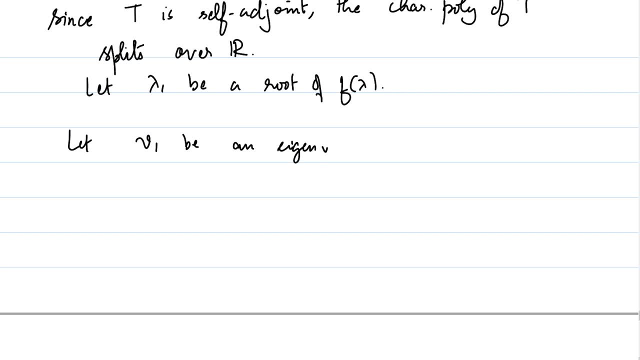 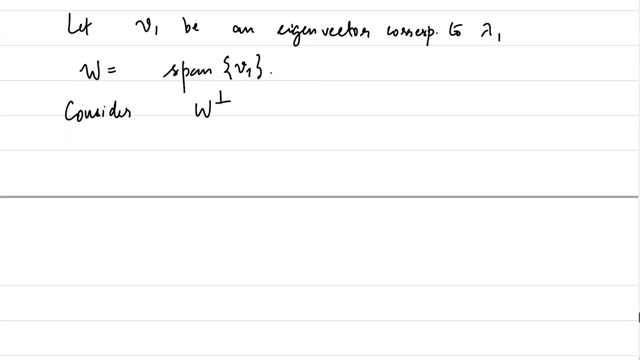 So let v 1 be an eigenvector corresponding to lambda 1.. Let w be the span of v 1 and consider w orthogonal. We notice that T and T star both are invariant. sorry, w orthogonal is invariant under both T and T star. 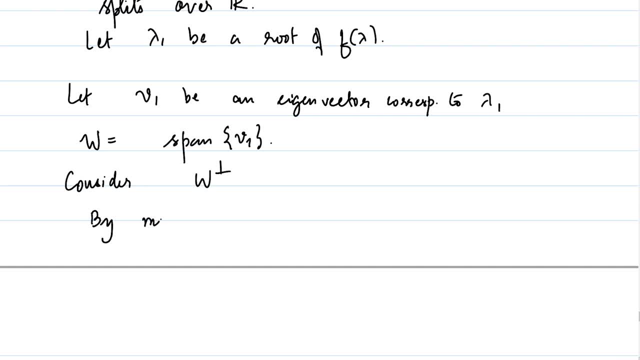 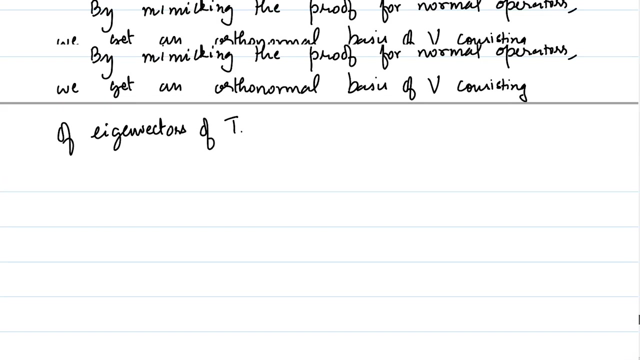 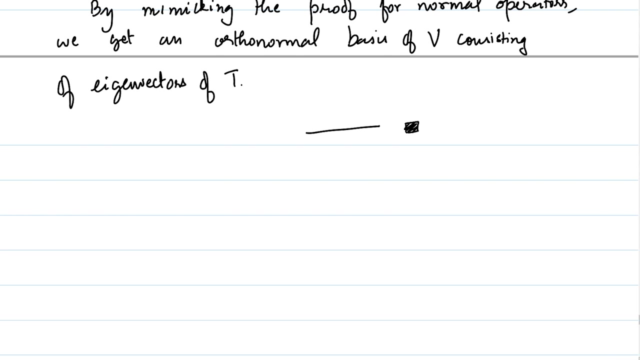 And by mimicking the proof for normal operators using the induction hypothesis, we get an orthonormal basis of v consisting of eigenvectors of v. Just say that it should go back to the proof of the spectral theorem for normal operators. 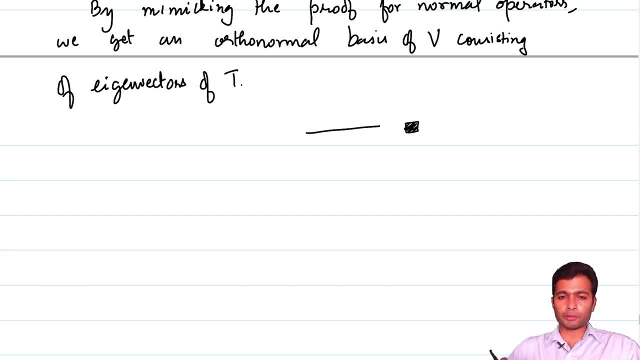 from the case when the induction hypothesis came into force. the proof is going to be exactly the same. Finally, getting hold of. finally, we will be getting hold of an orthonormal basis of v. it consists of eigenvectors of the self-adjoint operator T, And with that, 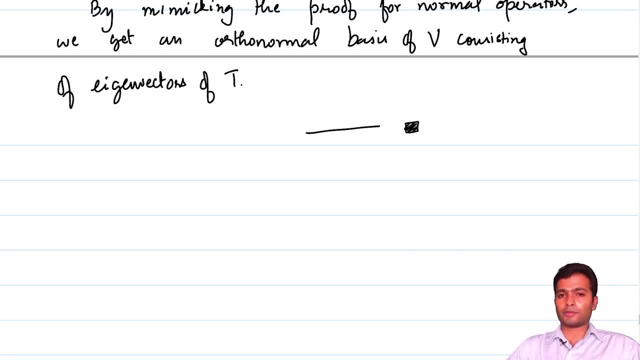 that will be the proof, completion of the proof of the spectral theorem for the self adjoint operators as well. So, even though I did mention that linear, the normal operators and self adjoint operators are quite special and not many operators are, most operators do not turn out to be normal.